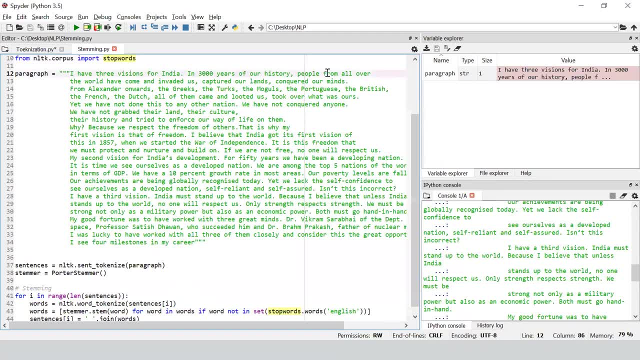 this kind of words, something like this: off from right or the and our of them. this kind of words are repeated again and again throughout this particular paragraph And this word does not actually play a better role. actually play a better role when we are, when we are solving different kinds of applications with respect to positive and negative sentiment analysis, because of 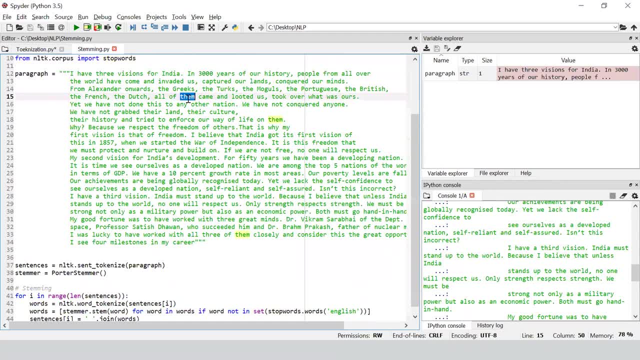 the them does not actually specify a much value in that particular sentences, right? So stop words helps us to remove this kind of words. So once we apply stop words in this particular paragraph, it will remove all this different kinds of words that we have. 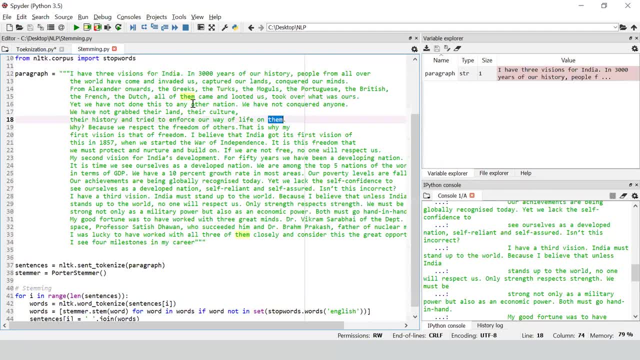 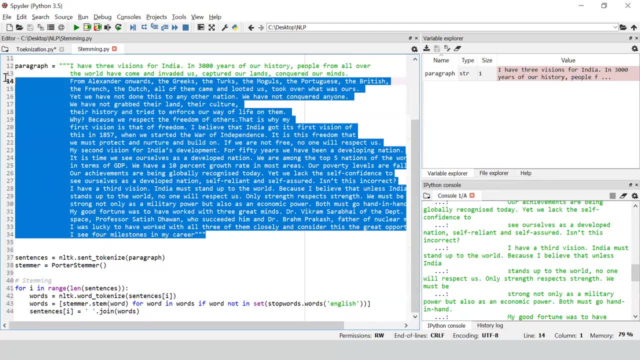 Words. that actually does not put much value on this particular scenario or application scenarios. we do apply stop words and try to remove this kind of words. okay, but before that, again i'm going to what, for the first step, that i always told you that i have to convert this paragraph. 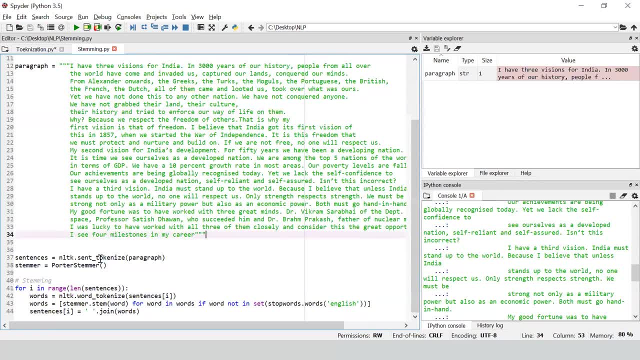 into sentences. right for converting this paragraph into sentences. i'll be using a function which is called as sent underscore tokenize, so once i execute this, you can see that i'm having all my sentences over here. it will take some time because it is a bigger paragraph and i have you. 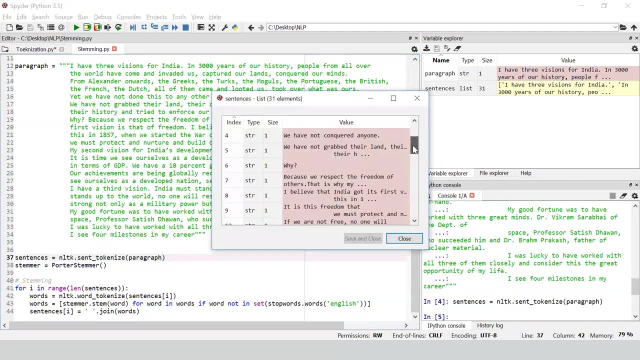 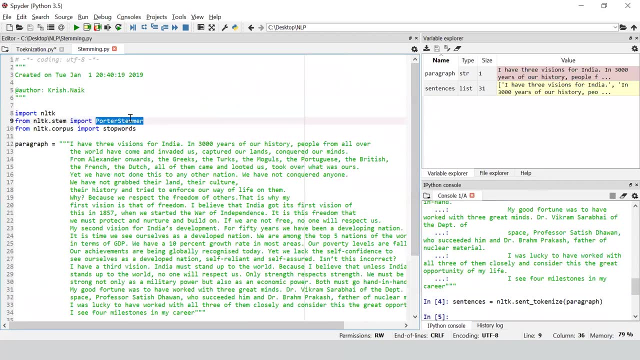 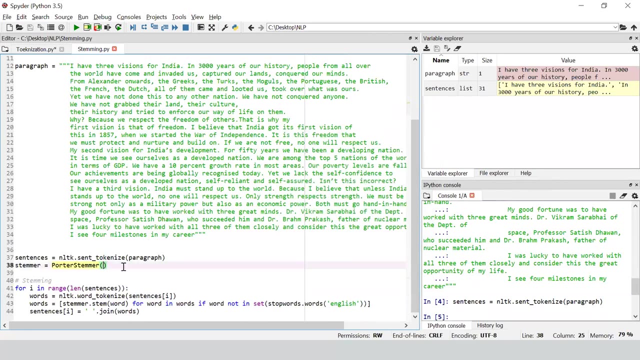 can see that 31 sentences that you can see over here right now, before applying then. then then the next thing is that i have imported a library which is called as porter stemmer, which was for stemming purpose, right? so this porter stemmer, i'm going to initialize it and i'm going to create an object of. 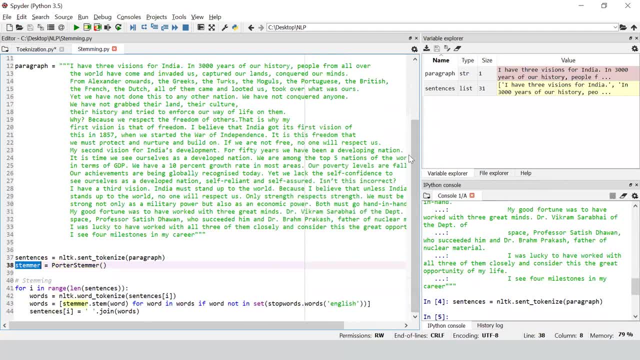 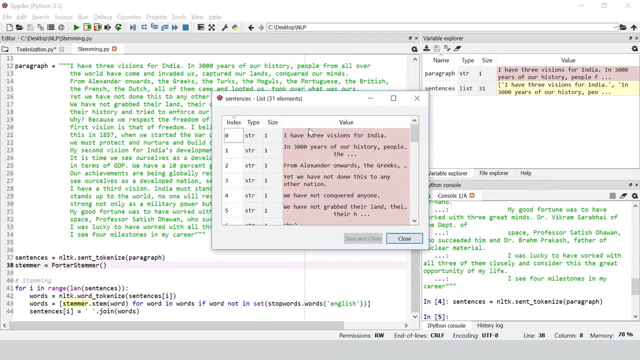 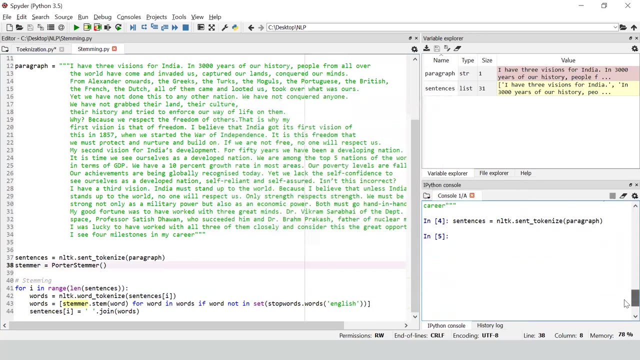 that that is stemmer. i've renamed it to stemmer. now what i'm going to do is that, for each and every sentences i'm going to apply, going to remove those words that are present in the stop words. if you want to see the list of stop words, what you have to do is that you just go to its console. 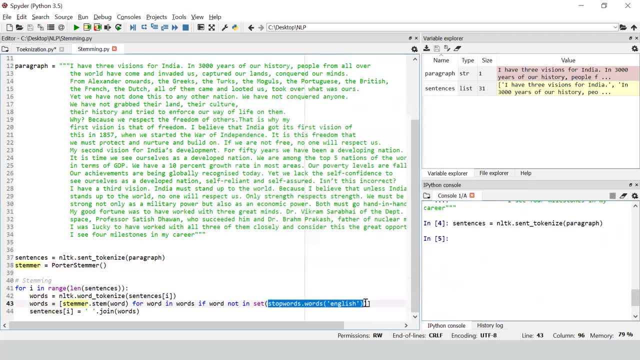 and just execute this particular statement, that is, stop words, dot words, and I want all the stop words with respect to the English language. once I execute it, you can see that there will be a huge list of stop words, which actually does not put much value in a paragraph when we are doing some. 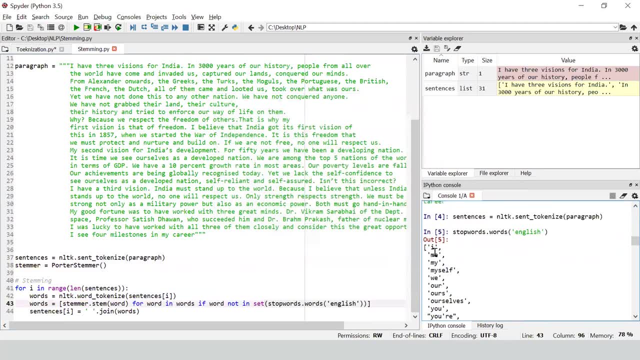 applications like positive and negative sentiment analysis, so you can see some words like I, me myself, we, our, ours, ourselves, you, you are, and all these words are basically stop words. right? the best thing about stop word is that you also have stop words in different languages, right? so if, if I go and 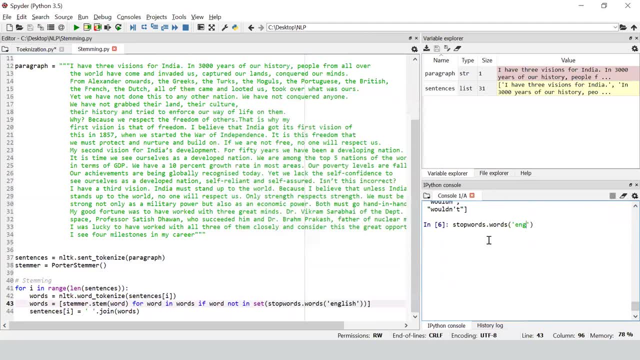 execute the same thing with different language like French, I'll write it as French. let's see whether we have any stop words for French, if I just execute it. yes, we do have some stop words of French, right? similarly, with respect to this, I may also have some stop words with different, different languages, like. 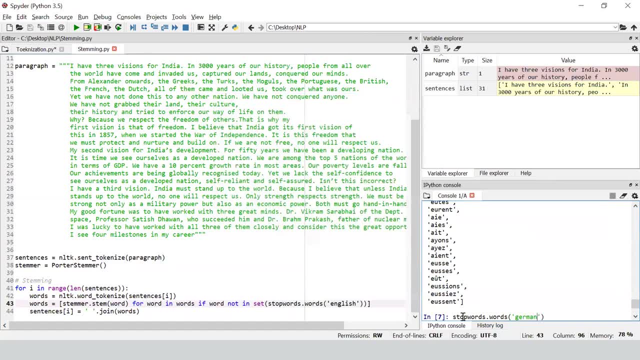 Spanish, or just let me write German. okay, if I execute with respect to German, um, you can see that there are also words with respect to German, right, so there are a lot of languages. the stop words, actually, you know it is present, and these all are present in that, inside an LTK library. so this analytical library, 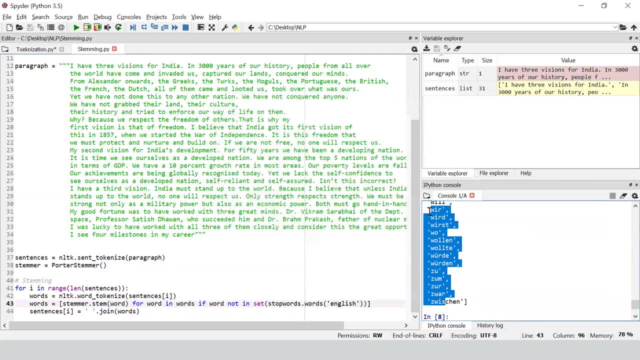 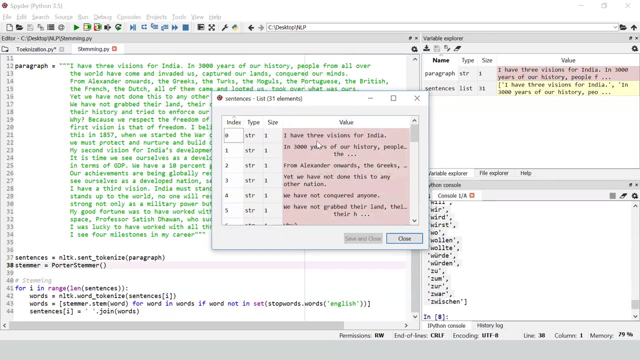 can be handy when we are doing text processing with respect to the other other other languages also. so, first of all, i have actually imported stemming. now my next step will be that whichever words, whichever words are actually present in the stop words, i'm going to remove those words from the sentences. right, that is the first step. then, after removing those, 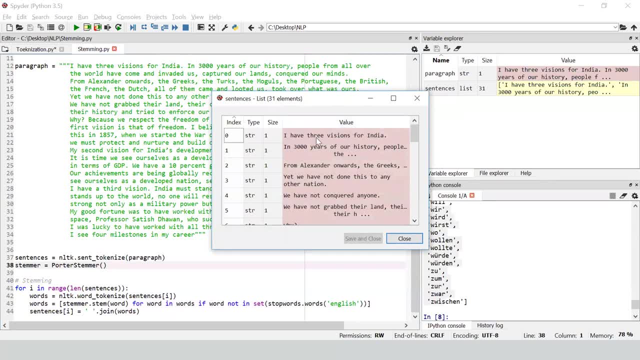 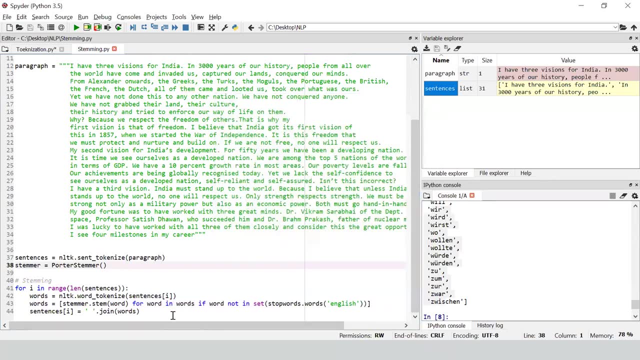 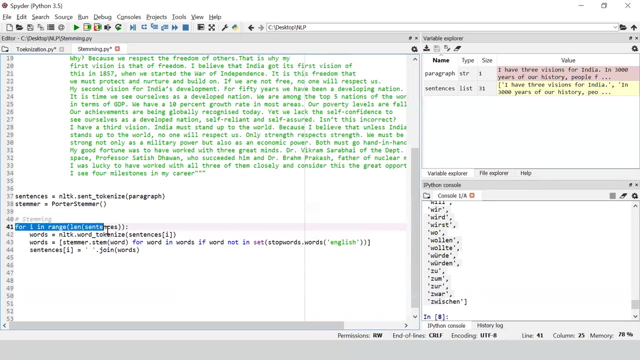 stop words. i'm going to do the stemming for each and every word by using this portal stemmer or the stemmer object. so it will be a very interesting code. you just see the code focus on this particular line for stemming. what i'm writing is that i'm writing. i'm putting a for loop on all these. 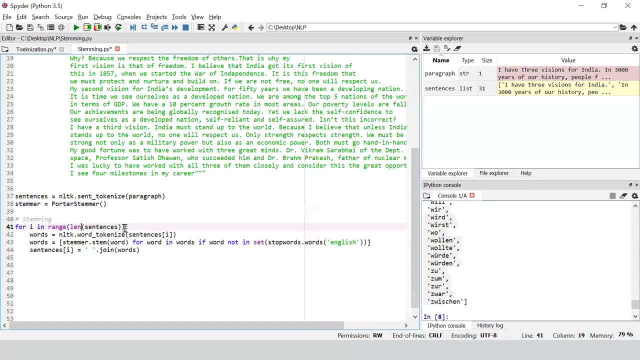 sentences. so i'm putting a for loop on range of length of sentences. my range of length of sentences around 31, so basically my range will be between 0 to 31 for each sentence. first of all, i'll do a word tokenize. word tokenize basically will convert all the sentences into words. 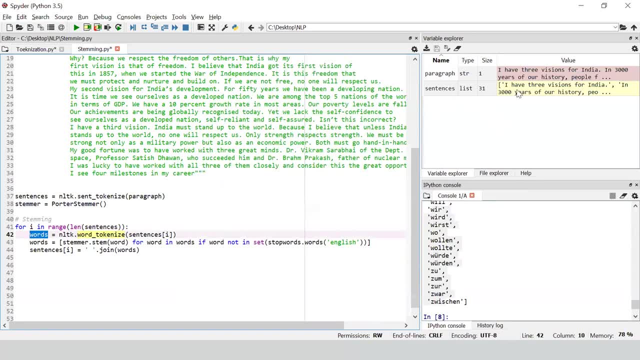 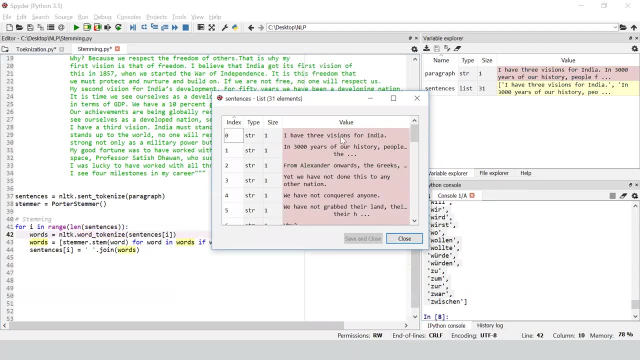 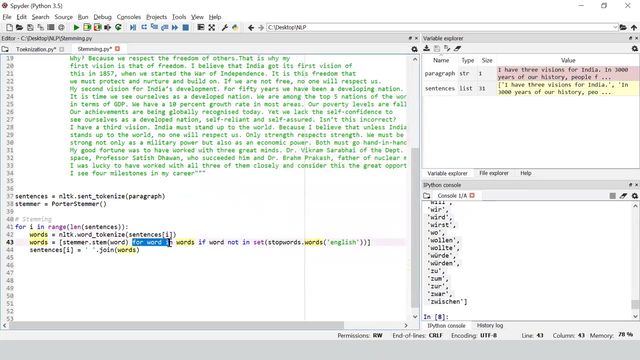 so this words will be a list of words from each and every sentences, right from. if i just take the first sentence, it will be one, two, three, four, five, six words. right then. after that, what i will do is that i will just write a for loop saying that, for words in words, for word in words. so basically this: 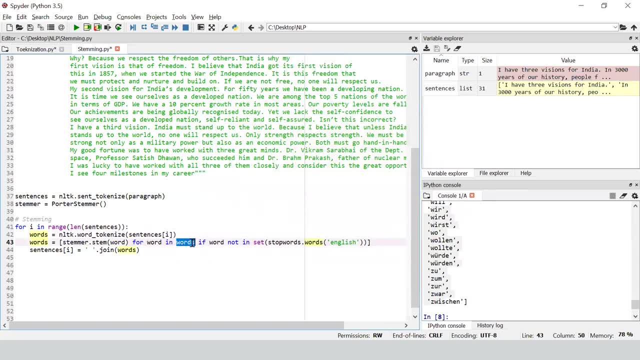 words is the list of words for each and every word. i'm going to, you know, iterate and i'll write a. i'll write a condition which says that if word not in set stop words, dot words of english. the reason why i have used set set actually helps us to take the only the unique stop words in the english language. so 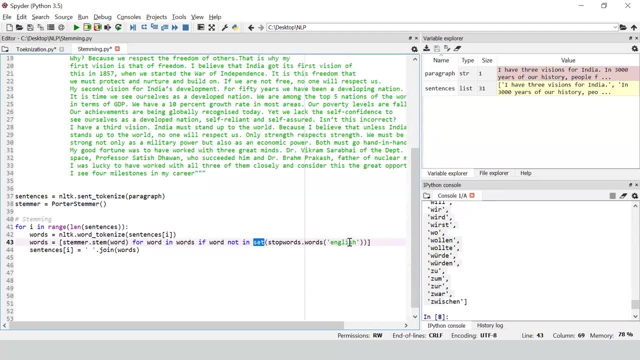 that unique uh set of words stop words from the english language will be compared whether that word belongs to this or not. if it does not belong, then only it is going to go and do the stemming, and stemming will be done by just writing this object. that is stemmer. 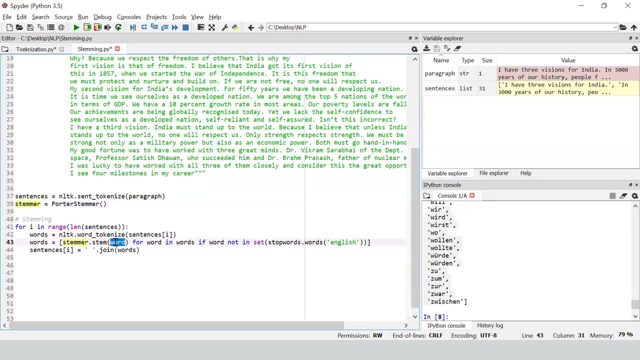 okay, dot stem, and then i'll put the word over here. so if there is a stemming to be applied in this word, the word will get stemmed right and this, this, this whole thing is basically called as a list comprehension right now. you see, in list comprehension i'm just basically putting a for loop. 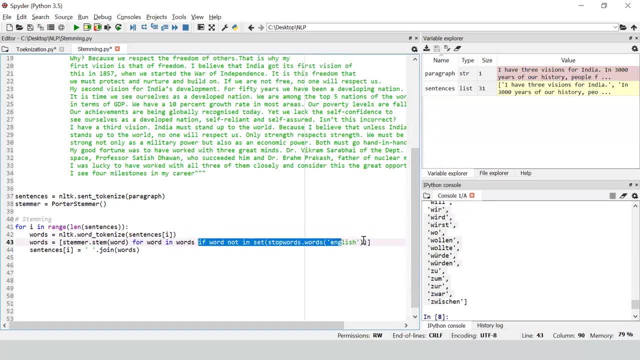 and then i put the condition if that word belongs to the stop words or not. if it belongs to the stop words, i'm going to remove it. otherwise i'm going to do the stemming process on that particular. after i get the list of words, i am going to join that words and convert back. 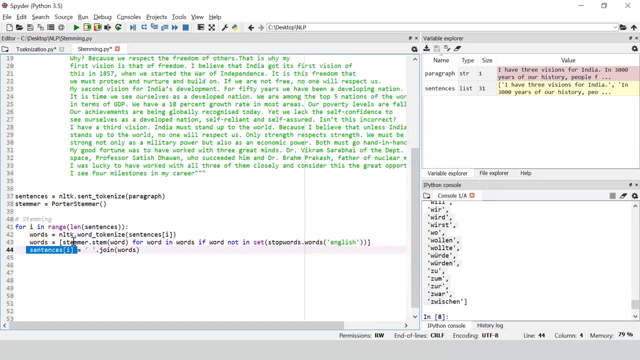 into the sentence, right? so i'm first of all what i'm doing. i'm taking the sentences i'm tokenizing into words, then i am applying the stop words on that word. if that stop words, if if the word is present in the stop word list, then what i'm going to do? 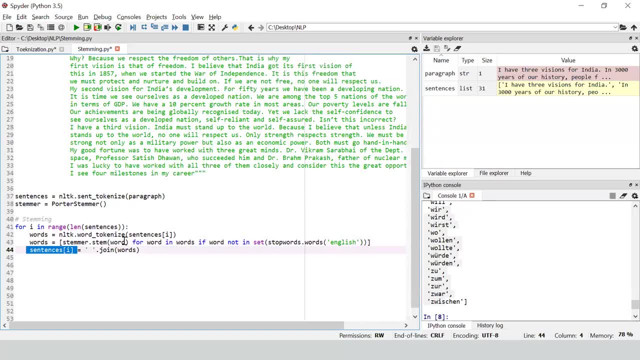 i'm not going to take that word. instead, if it is not present, i'm going to take that, i'm going to apply the stemming onto that and, finally, i'm going to join that into sentences. so once i execute this, you can see that i think it will give you an error, because i have not. 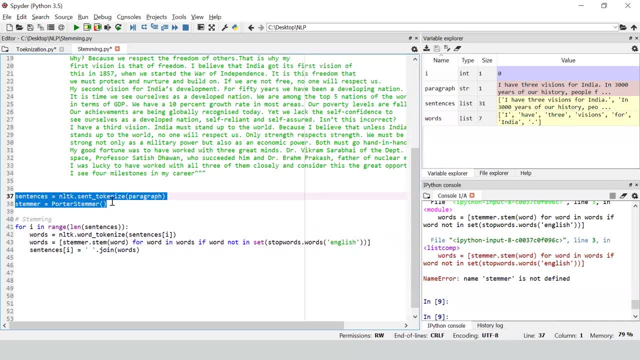 executed this two line of code, so let me just execute it. i think i have executed the sentence underscore tokenized, but i have not executed the port stemmer. let me create an object with respect to port stemmer, so stemmer is the object that is created. i'm going to execute this three line for.